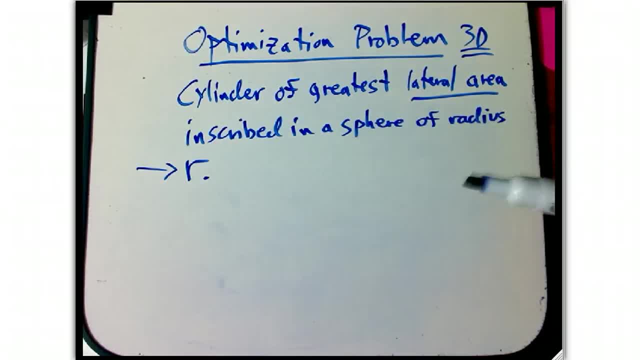 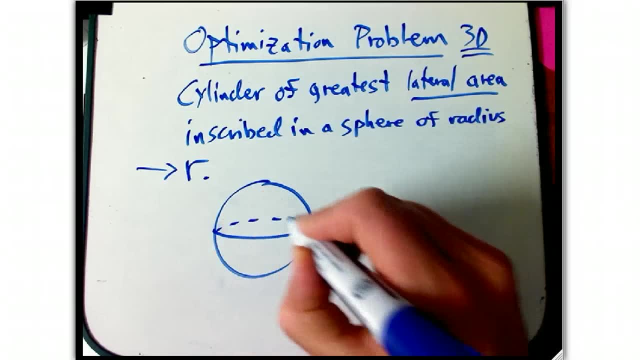 the lengths are all going to have to be some number times R and that's going to be a check. Here's the picture. Here's the 3D picture. Here's our sphere. It's not too hard to draw. Here's the cylinder. It's not too hard to draw. 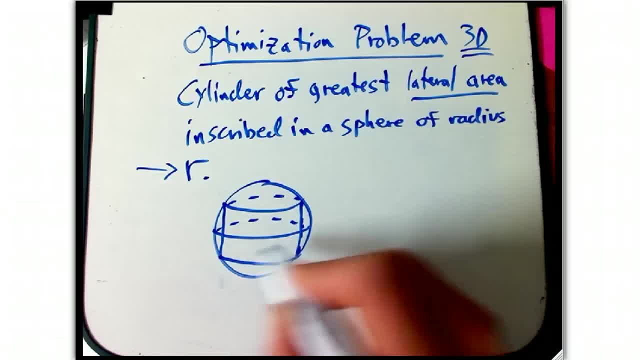 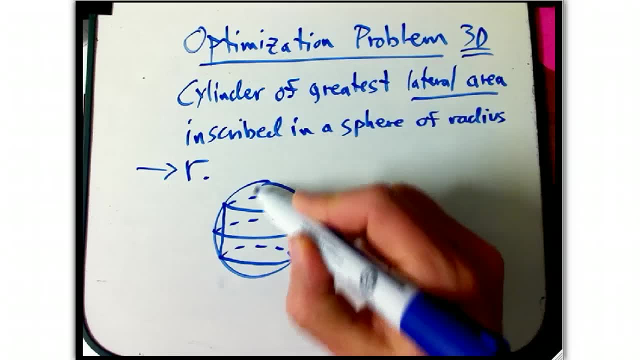 We're not going to do anything where it's really hard. So there's our cylinder, and it could be really skinny. Maybe it could be actually really skinny. Well, that might not have the best surface area because it's really tall, but it's pretty skinny. 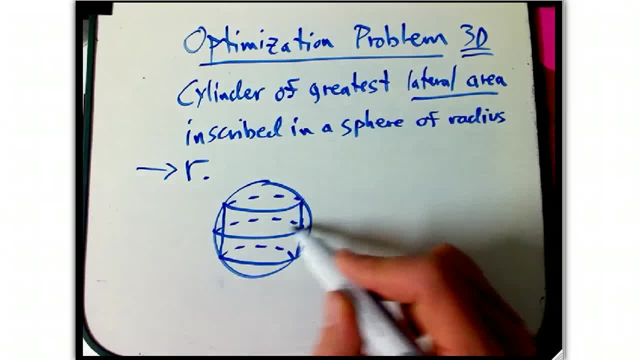 Or it could be really wide, but then it'd have to be really flat. That's probably not going to be the best either. So it's probably an interesting optimization problem in the sense that the endpoints aren't going to be the answers. No, the endpoints can be the answers sometimes. 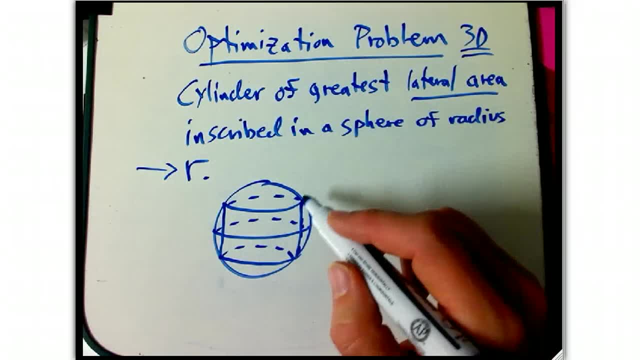 Well, it's probably not here. The key here, though, is that there's really a 2D picture hiding. The key here, though, is that there's really a 2D picture hiding. The key here, though, is that there's really a 2D picture hiding. 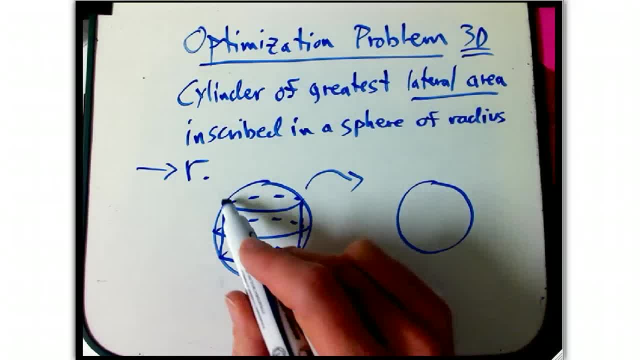 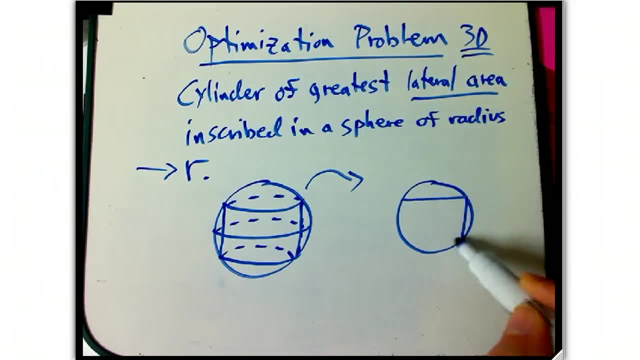 And that's just a cross section. Just slice it through with the plane of this board here, Just slice it through with the plane of this board here, And you really just get a rectangle. And you really just get a rectangle, And the key thing is that that's. 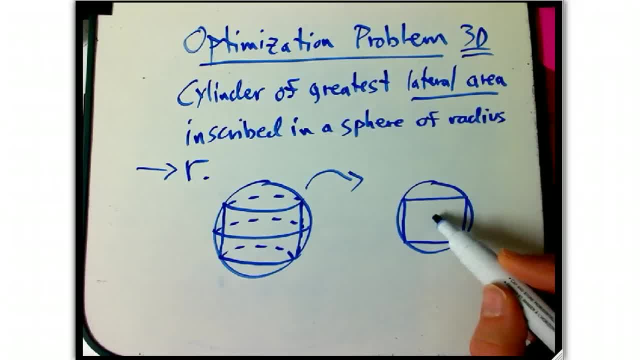 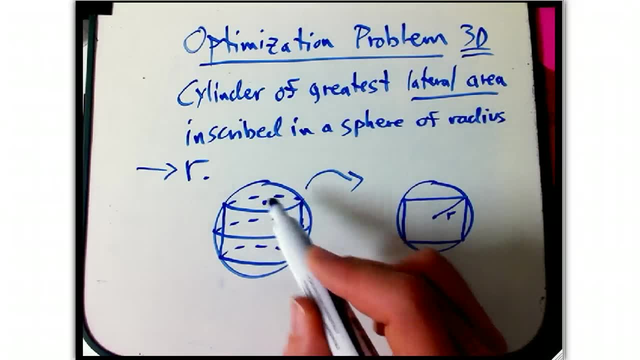 And the key thing is that that's that slices a circle. So that's a circle of radius r, And now I just need names for the width, And now I just need names for the width. Now, one thing that often confuses people is: 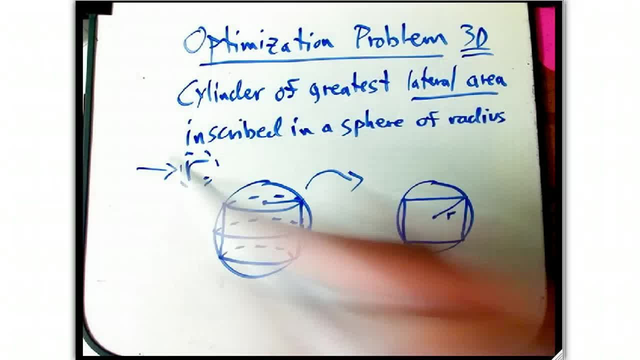 they want to use r for the width of the cylinder. Sorry, it's already the radius of the circle, So let's just use x. it's a horizontal in the picture. So let's just use x. it's a horizontal in the picture. 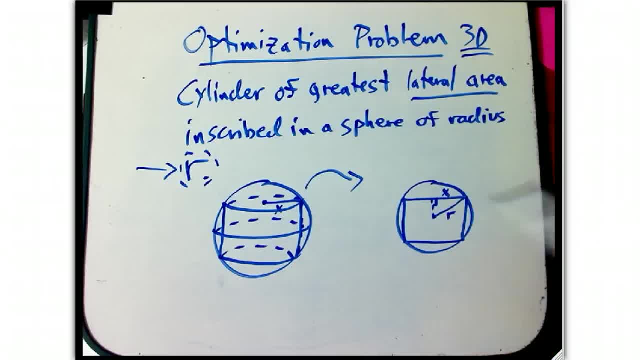 And that's just exactly x right here. Hey, that's an x and a right triangle. And what about the height? And what about the height? Well, you could use the full height, but it's going to be better if we actually just use this as y. 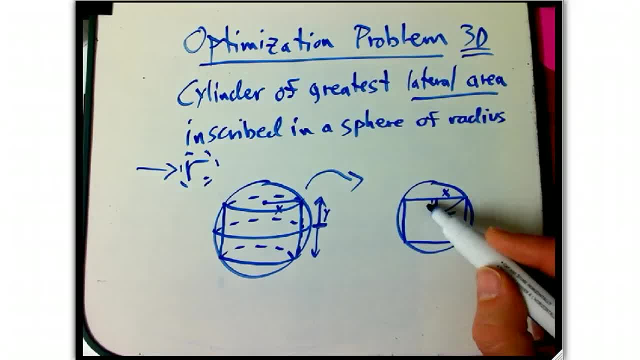 but it's going to be better if we actually just use this as y, And then the whole height is going to be 2y, So that's y, right there. Hey, I've got a right triangle. That's a constraint, right there. 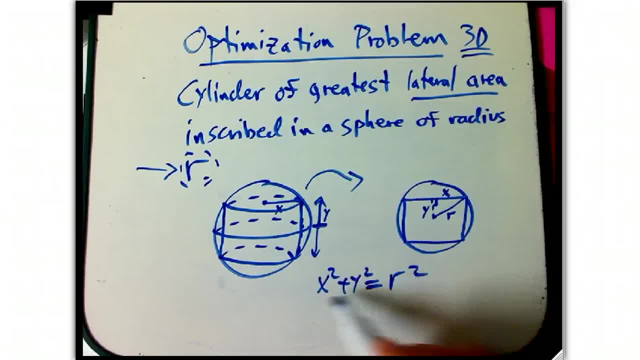 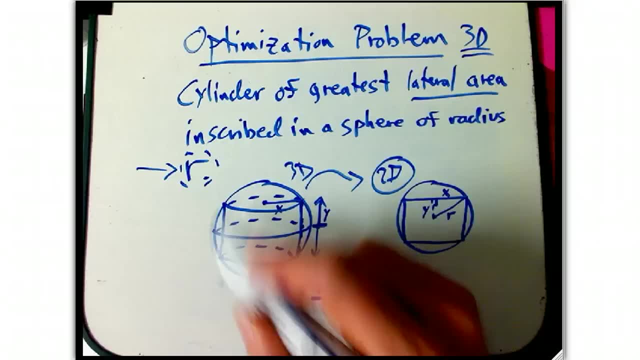 So we've discovered our constraint: equals r squared, And the key was taking a 3D picture and reducing it down to a key 2D picture. This 3D picture is just this picture revolved around the middle of it, And that's very common. 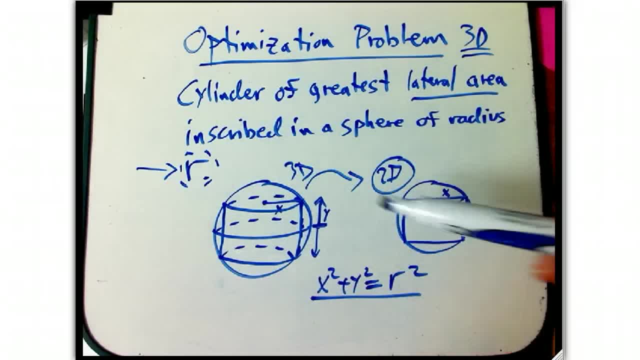 Most of the 3D examples. well, I think every 3D example we would do in this class, in A-B, Calculus would be symmetrical in some ways, But it's secretly really a 2D problem. Okay, so there's our constraint. 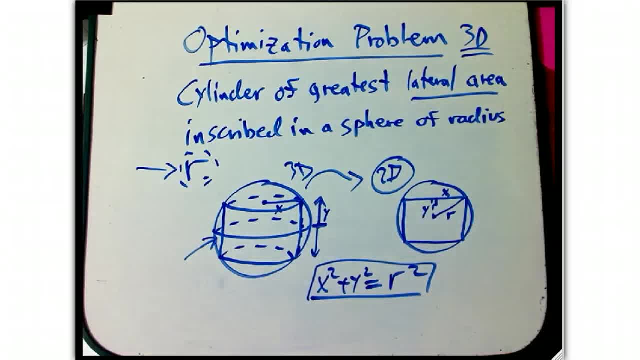 What's our objective function? Well, that's the one place where we really do use the 3D nature, but just in terms of memorizing a formula. What's the lateral surface area? Just the sides of this guy? Well, it's 2 pi x. 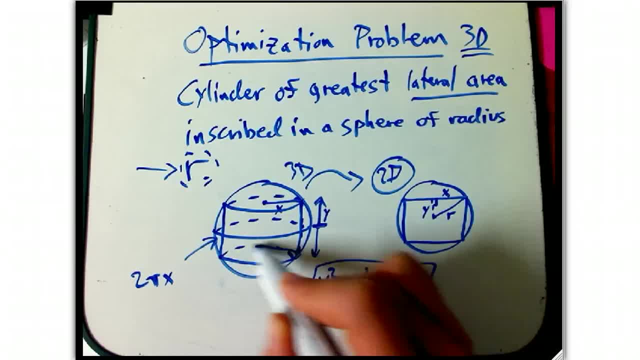 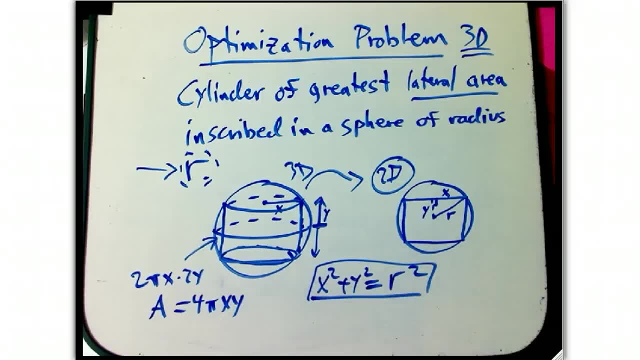 because, remember, the x is the radius of the cylinder, so that's the circumference of, say, the bottom times the height, which is 2y, And so the surface area, the lateral surface, is 4 pi xy. Okay, Almost got it down to where we want. 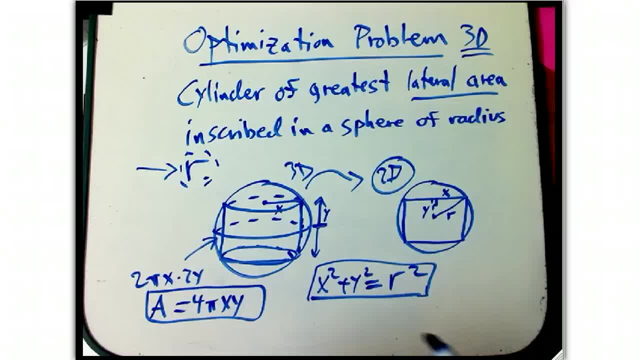 We've got a constraint, we've got an objective function, and I've been emphasizing the last couple days that you really want. this is the stage where you want to be careful about your bounds as well, And it's very simple: Just x and y. 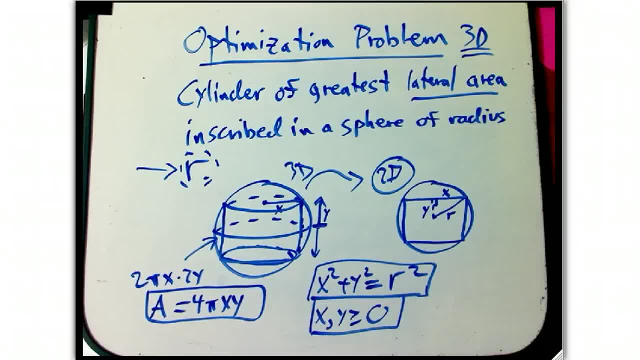 have got to be non-negative numbers. They're lengths, And we'll see how that comes into the rest of the problem. So that's a really important thing if you're going to be careful about this stuff. Alright, now I'm going to erase it all except for. 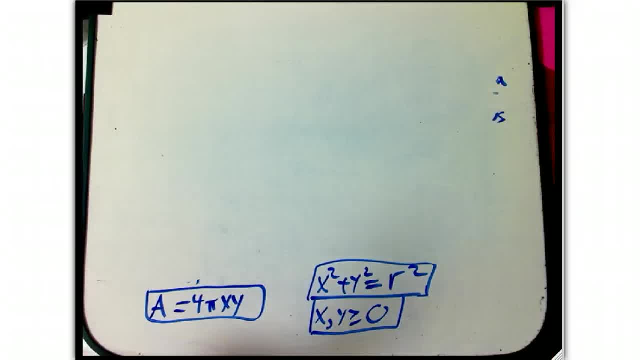 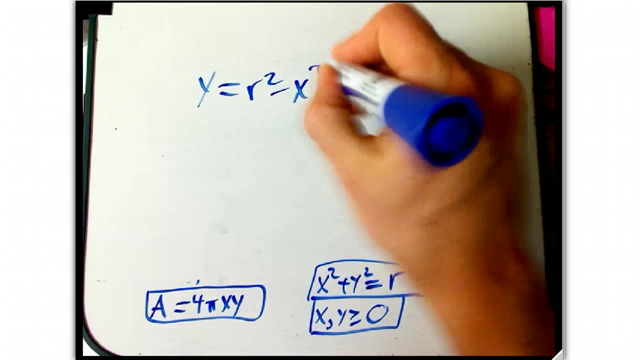 that crucial data. Okay, Let's solve the constraint. It looks very symmetrical here. x and y come in symmetrically and these inequalities that come in symmetrically, So it doesn't really matter. Let's go ahead and solve: y squared is r squared minus x squared. 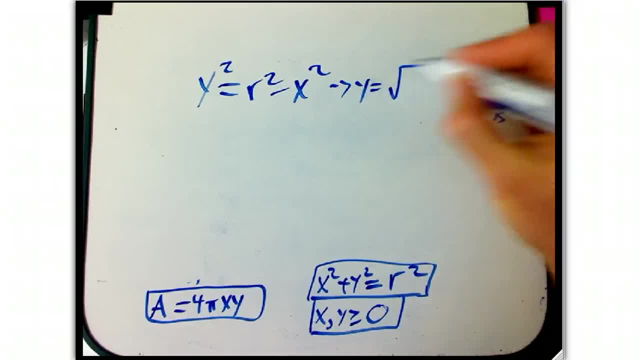 So y is the square root of r squared minus x squared. We don't need a plus or minus, because we've decided that it's a length and we don't get anything from flipping stuff upside down. that's different, So that's going to be just plus. 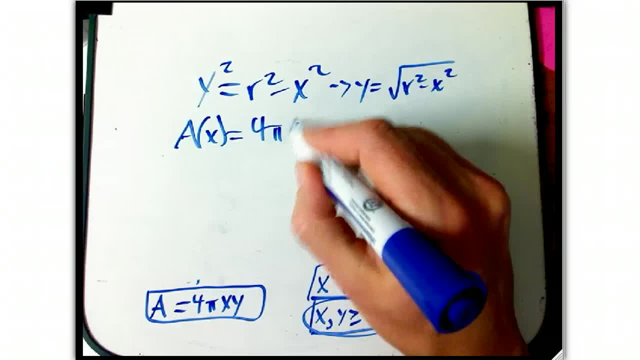 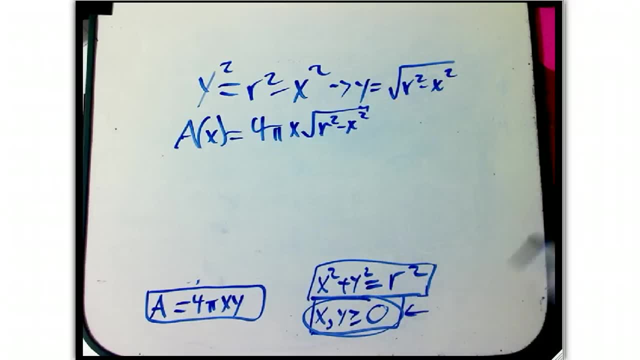 And so my a of x now is going to be 4 pi x root r squared minus x squared. And now is the time to take these sort of simple constraints and turn them into a boundary, an interval. thank you For, for x. well, x has to be. 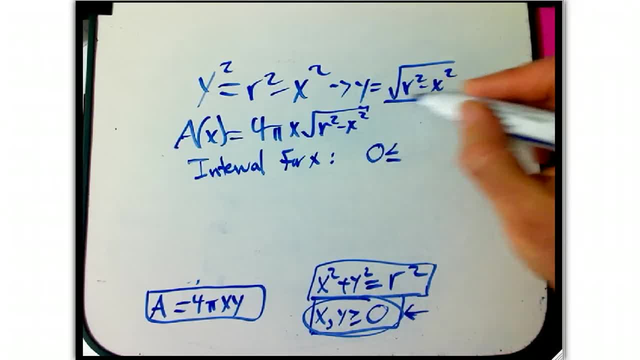 non-negative. And then if y is going to be non-negative, whoa that means? or if y is even going to make sense for this problem, the biggest x can be is equal to r, which makes sense If you look back at the picture. I'm not going to redraw it. 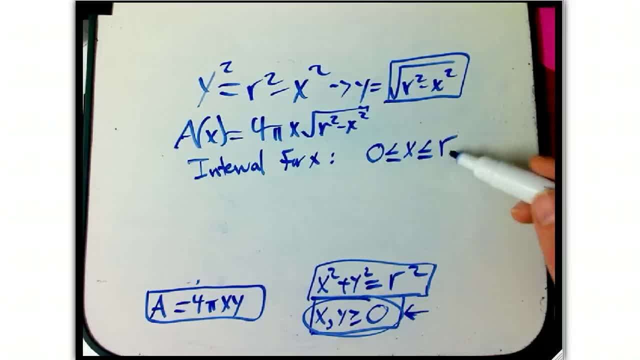 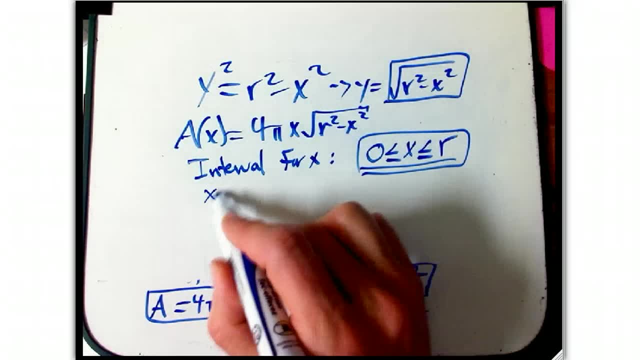 That's where it kind of becomes a pancake, And it's clearly not going to be the maximum, but that's going to be our interval. So one thing you can do very often is you can just check the endpoints right away. x equals 0, clearly. 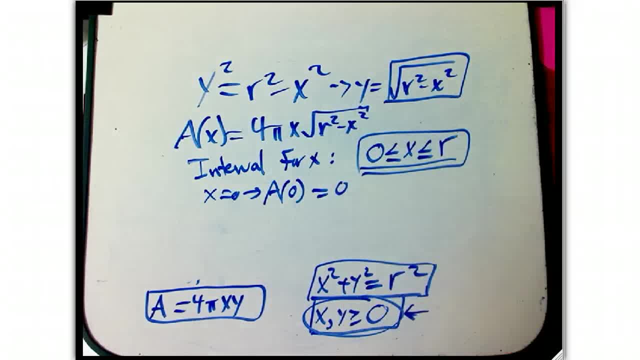 a of 0, this dies and you get 0.. Boring x equals r. a of r equals this dies and you get 0.. And that's because the long skinny pencil and the big pancake, they both kind of degenerate to 0 area. 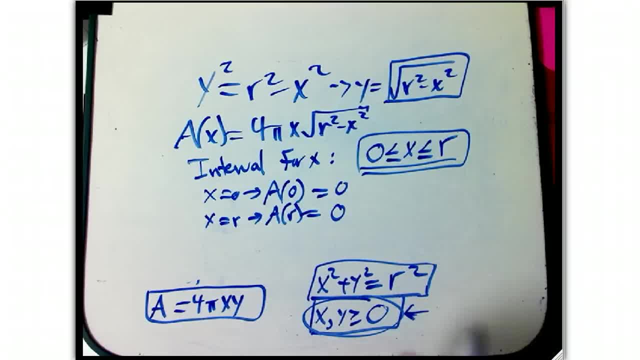 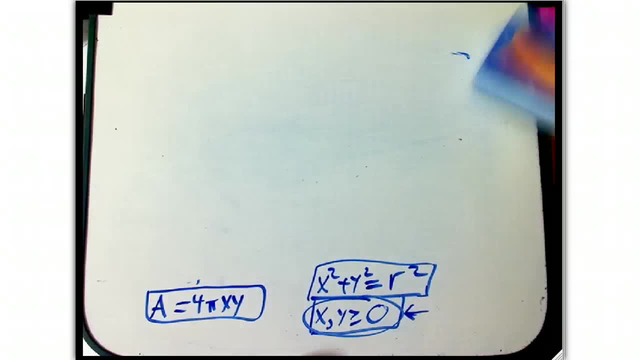 Okay. so alright, now we're going to need to take the derivative of that And I think I just need to redraw. The great thing is, you can always rewind, So don't be afraid to rewind. Okay, so let me write. write up a of x one more time. 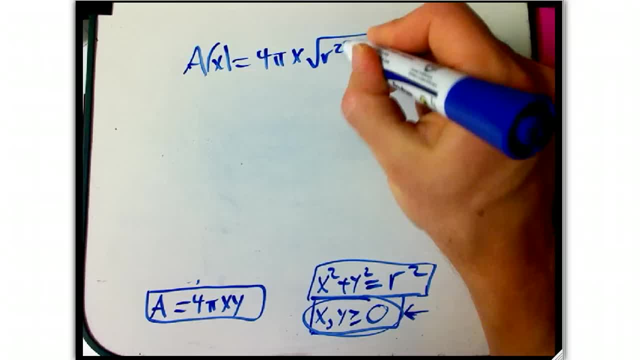 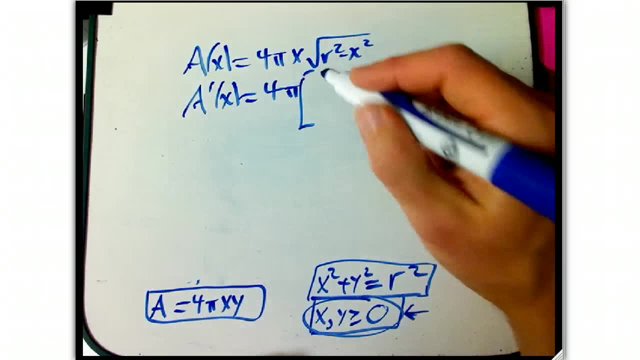 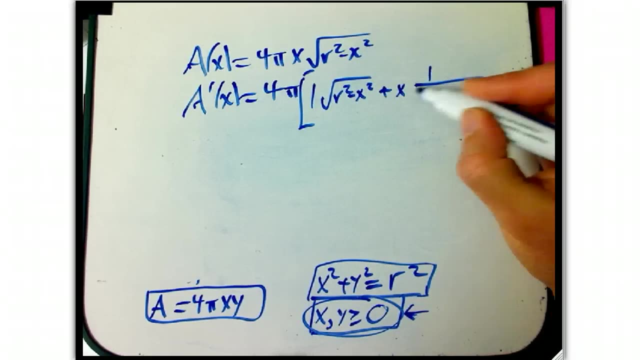 A little higher this time: 4 pi x root r squared minus x squared a prime of x, 4 pi is a constant. now we need the product rule, So it's all times 1 times the square root, plus x times 1 over 2. 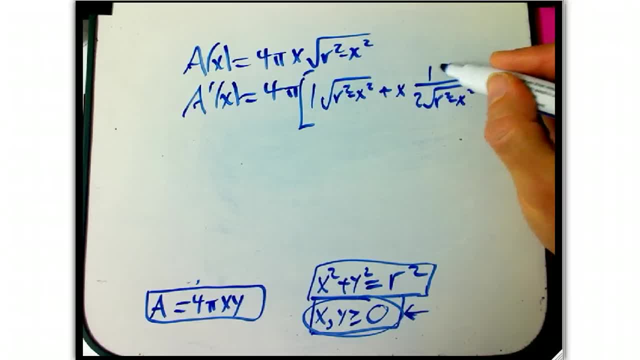 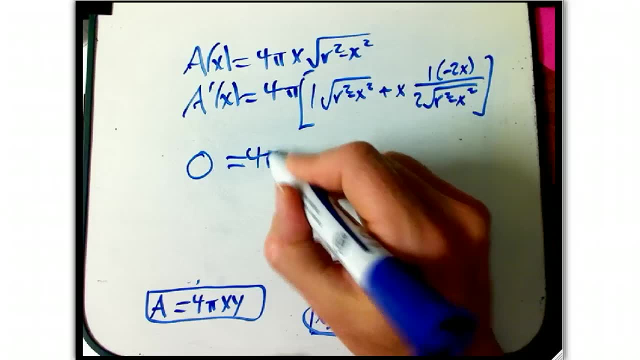 times the square root And then times minus 2x from the chain rule. Now I'm going to set that equal to 0.. So the 4 pi is very quickly going to be uninteresting. Now I'm going to put it over a common denominator. 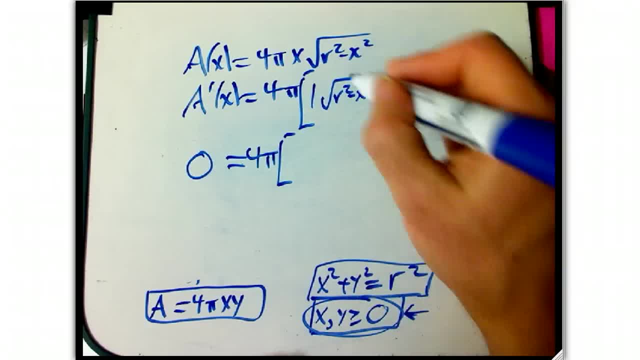 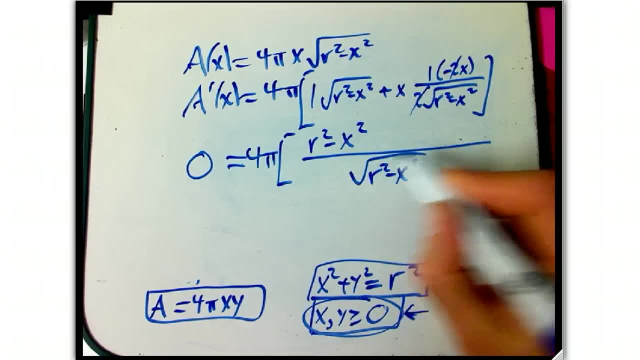 Although let's cancel out the 2's first, So putting this over a common denominator of the square root of r squared minus x squared, that bumps it up to a full r squared minus x squared, And then minus x squared. oh so that's just r squared.